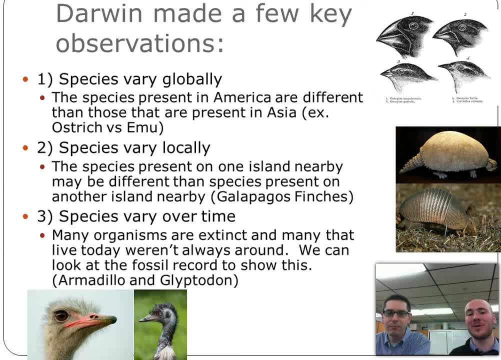 influential in Building evolutionary theory. But anyway, a few things you know is, first of all, around the world there are species that are different, species that look incredibly similar. Furthermore, and kind of separately, I guess within very close areas, depending on the terrain- 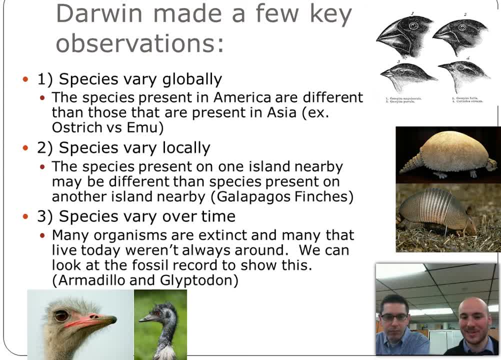 you can see that there are different species in different areas that are still pretty close by to each other. And finally, and Darwin. actually, I mean, this was back when we were first starting to actually look at fossils. Darwin caught on to the whole fossil thing. 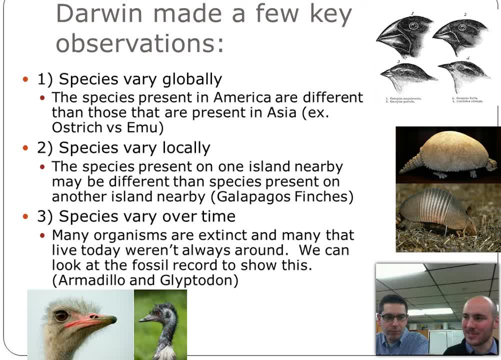 and noticed that, you know, life on Earth isn't always how or hasn't always been the same. What the. in fact, there were species that were on Earth at that time that really weren't in the fossil record, And likewise there are things in the fossil record that were not on Earth at that. 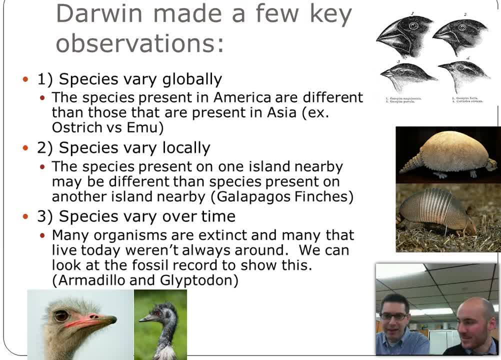 time- And this was controversial at the time- making these claims. Yes, absolutely controversial, because it was thought that all life on Earth had always been the same. There's the bell, There we go, But it was thought that all life on. 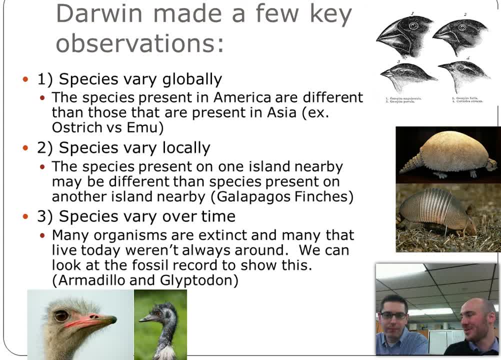 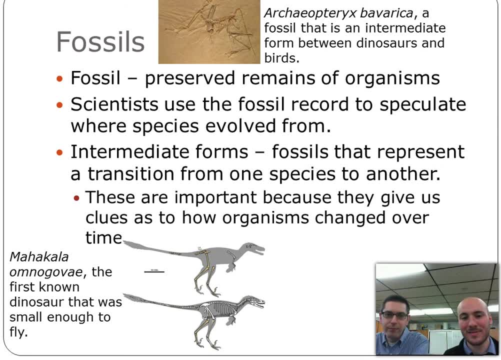 Earth had always been the same, no matter what. They didn't really even know what dinosaurs were at that point, So but anyway, we're going to address all these ideas in this little presentation here, But hopefully you guys know what fossils are. Mr Hillis knows what. 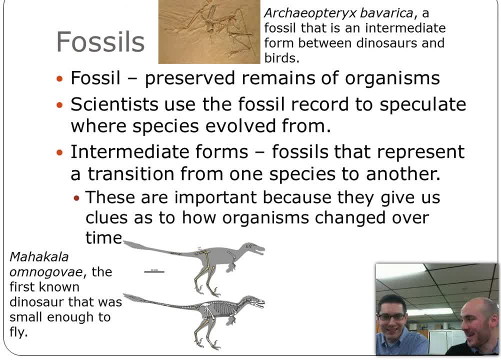 fossils are. I said I always wanted to be fossilized. It's a way to go. We'll talk about how that happens in a minute. But fossils are preserved remains of organisms and the reason why they're important for evolutionary theory is that scientists take a look at them and 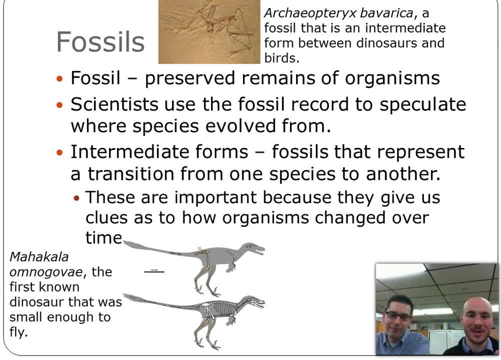 they use them to speculate where species on earth now, or even previously, might have evolved from, and they use particular fossils called intermediate forms quite often, and intermediate forms are fossils that represent maybe a midpoint between two species that we know exist, one in the past and one further along in time, whether it be a current species or even, you know, maybe. 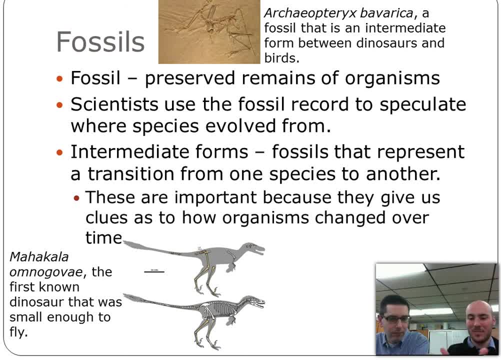 two dinosaurs that exist in separate time and they find a fossil that looks like it might be the midpoint between those two. really famous one up there at the top is called the Archaeopteryx. it's maybe the most famous intermediate form of all time. it is a dinosaur that also had feathers, but there's really no we. 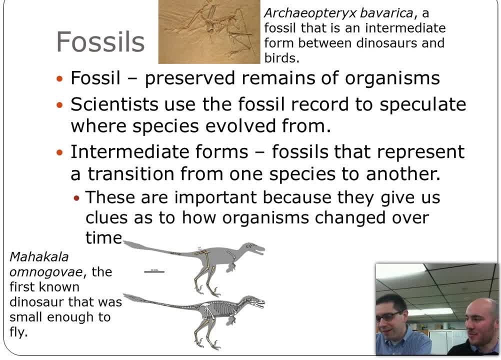 don't think it really could fly, but it's thought to be the intermediate form between dinosaurs and birds. so that means not all the dinosaurs might have died off and some of them could be present-day birds. there are some that argue that birds have a closer relation to dinosaurs than our current reptiles have to. 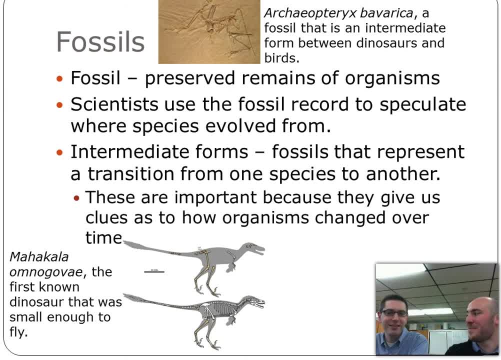 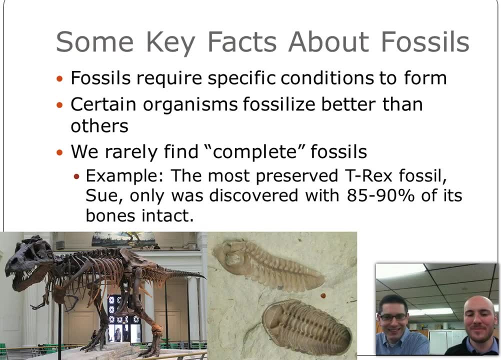 dinosaurs. we're gonna explore that actually in our next unit in a bit more detail. hey, maybe this unit we'll see, it'll probably come up in conversation- knowing my students, especially now that you've said that- but yeah, we'll talk, take a look at the heart and everything like that. but anyway, now there's some. 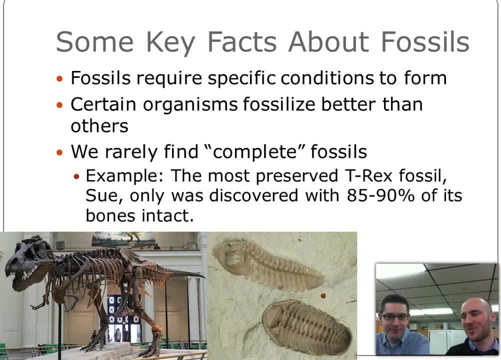 misconceptions about fossils that I need to set straight. first of all, fossils don't just form all the time. fossils need specific conditions in order to form. so let's say we wanted to fossilize mr Hillis here. well, you probably. you can't just let them lay out in the desert and hope he fossilizes. okay, you need to get. 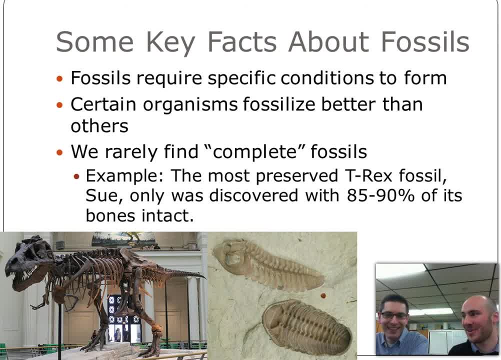 buried alive, basically, or buried almost immediately after dying. and I'm not talking about in a coffin, I'm talking about in a bunch of sediment. so, whether it be a mudslide comes through or a bunch of pebbles, or pebbles might even be too big like sand, something the same, really like mud and really fine silt. 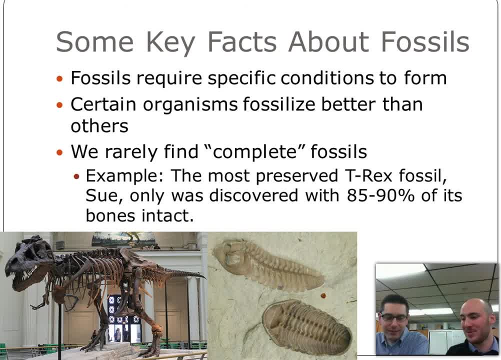 yeah, basically, and liquid, really specific sediment to do that, and it can also happen in ice, but needs to happen very fast really. so right there, that sort of eliminates a lot of things from being fossilized. I mean, it's it's really rare that things get fossilized, so if you 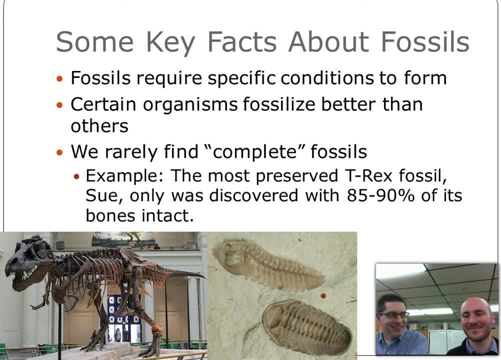 take me to a muddy area. I should be nervous. no, so also. certain organisms fossilized better than others, not to mention certain body parts fossilized better than others. so when we do make our Hillis fossil his skin and you know that that won't fossilize as well, say your bones, okay. 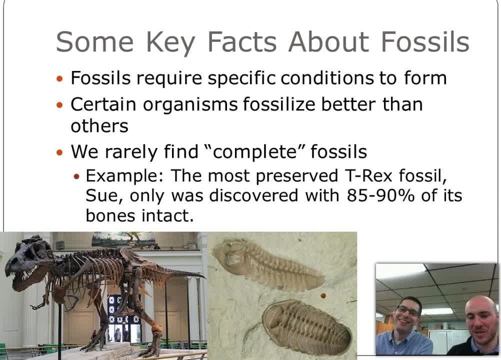 this is starting to sound really creepy, but this is why things with shells tend to fossilize really well, or with dinosaurs, we only really see their bones. we don't see any of their scales or anything like that, and furthermore, you might not realize this, but we rarely find complete fossils, even sue, which is 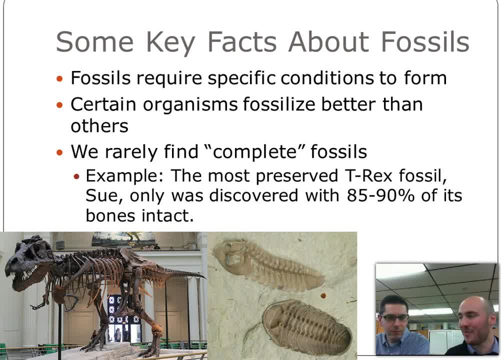 maybe the most famous t-rex fossil, which you're very lucky to have only just down the road in the Field Museum in Chicago. an exciting place to spend the weekend- yes, free for teachers, by the way- but it was only discovered 85 to 90 percent complete, and it is the most complete t-rex. I don't know about the 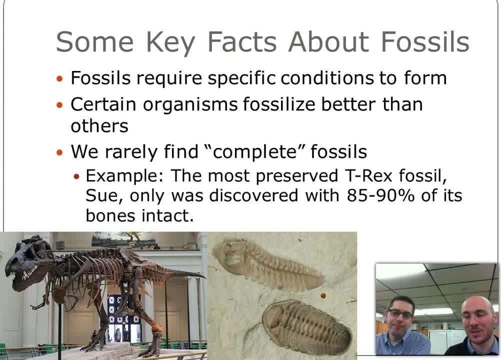 most complete dinosaur, but most complete t-rex. it's much more complete than most the other fossils we have. now you might ask yourself: okay, well, if we never have a complete fossil, how do we know what they looked like? well, you can compare other fossils, see, if you can like. let's say, part of Sue's tail is missing, maybe. 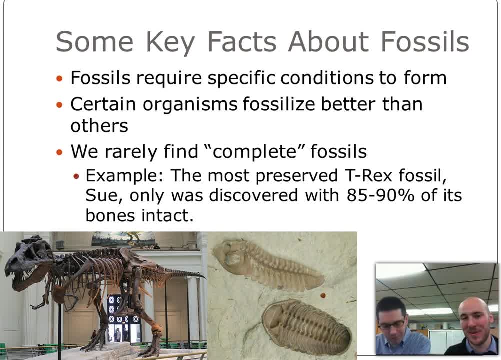 that part of the tail is missing. maybe that part of the tail is missing. maybe they're in another t-rex fossil. they're also- people are just very good at their major experts at this stuff- that like they know, they know dimensions of bones like inside and out, and I do know- yeah, that's not our area of expertise, but we 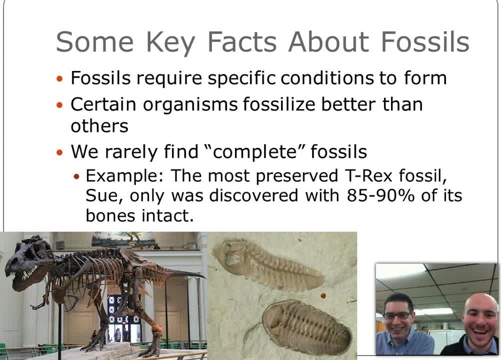 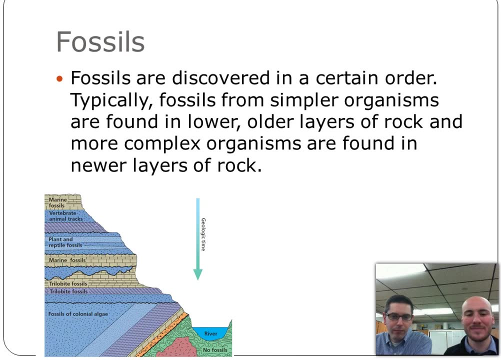 have an area of expertise. that's true, but anyway, now some say there are gaps in the fossil record. but maybe when there is an understanding of these three points, it kind of explains why there's a gap in the fossil record. so anyway, now another thing about fossils that doesn't have to do with how they're. 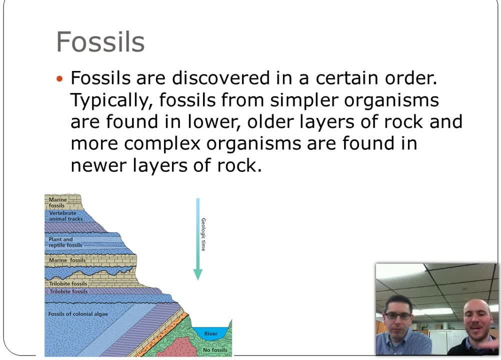 formed, but fossils, you know they get buried over time. you can probably accept that older fossils are gonna be deeper down in the rock because more Rock gets piled out over time, okay, well, when we dig up fossils, things that are thought to have evolved later, such as vertebrates, they're found way up at the 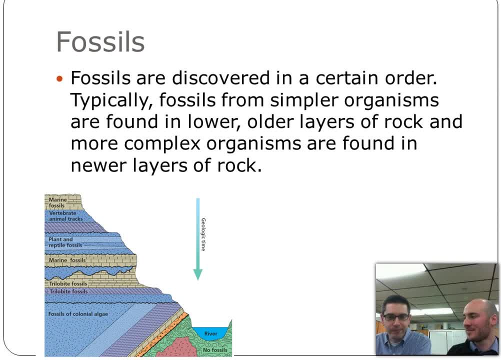 top, as opposed to things that very ancient evolved long, long ago, so like way, way down in the earth, and they're found way up at the top, as opposed to things that very ancient evolved long, long ago, so like way way down in the rock layer. we only see algae and bacteria and we see nothing else. we 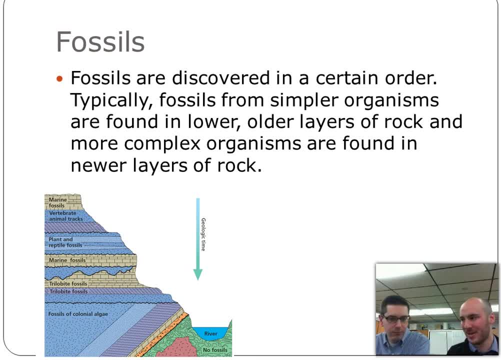 don't see any mammals. we don't see even any like fish or worms- worms probably don't fossilize very well anyway, but you only see stuff that evolved a long, long long time ago, and even to a point where you get deep enough down, you don't see. 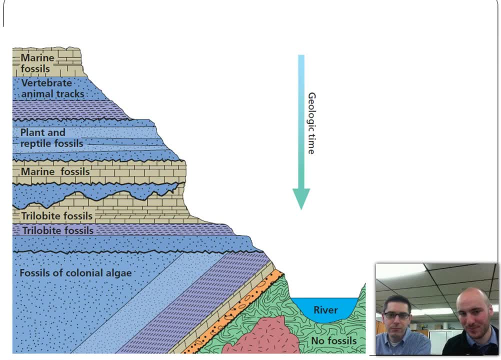 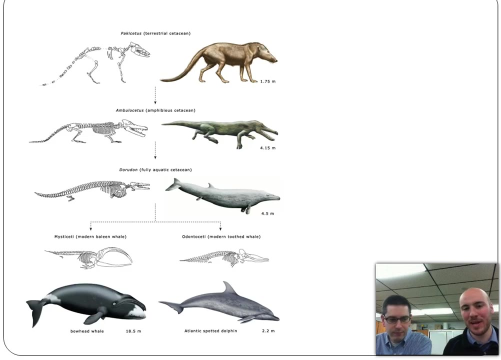 any fossils. here's a larger picture of what that looks like, just so you can take a at where we generally find things in the rock layers. so, as you could see, we find really Reptiles more recent than, say, mammals. Yes, and here's some transitional forms between a. 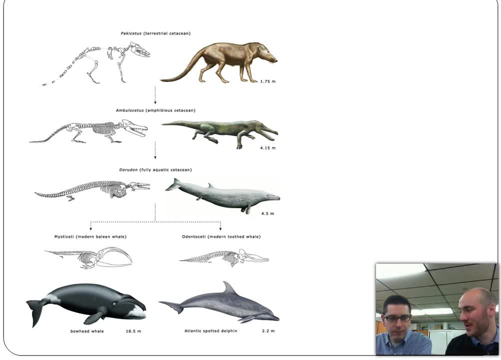 What's thought to be the terrestrial ancestor of whales- whales or mammals? We're gonna get into this one in detail in class, but I wanted to show another transitional fossil example. 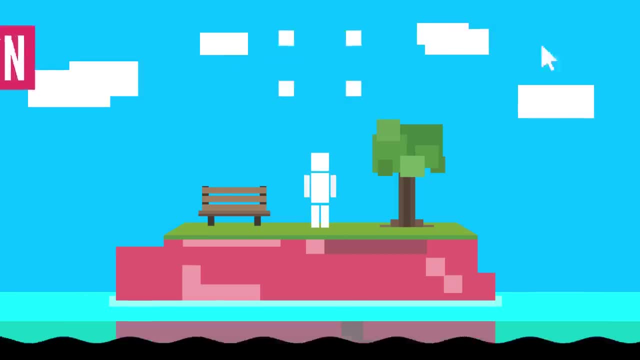 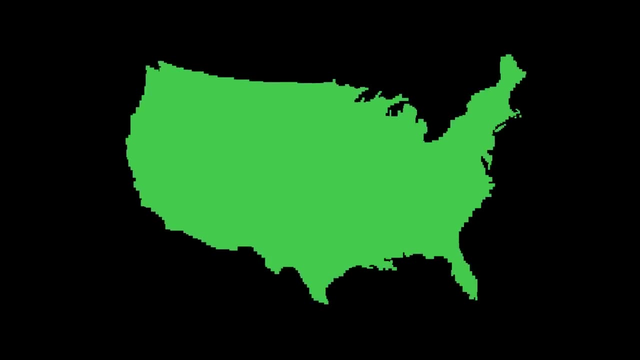 Hey there, Welcome to Life Noggin. The world uses nearly countless amounts of oil every year in one form or another. The United States alone has been consuming a total of over 7 billion barrels of petroleum products a year, or around 20 million barrels a day. in recent times. This 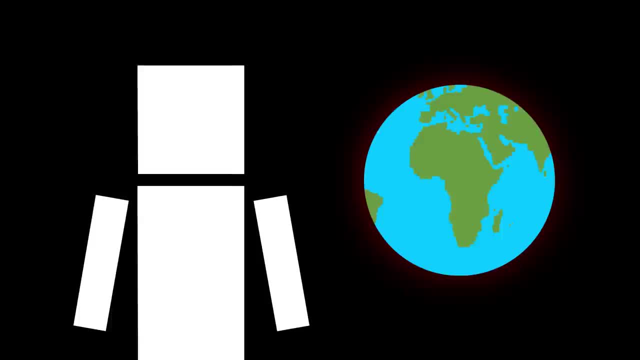 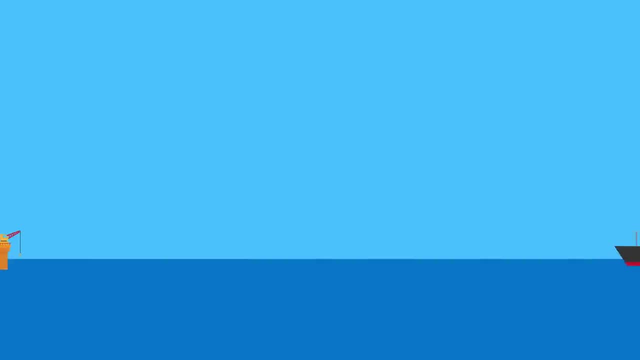 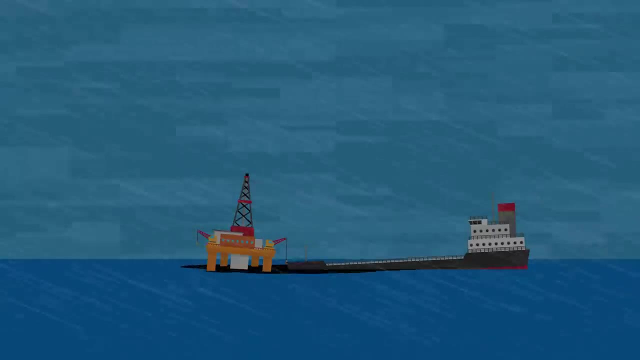 reliance on fossil fuels has its own host of long-term environmental problems, but when you have an oil spill, you create another world of issues. Oil spills can happen for a variety of reasons, from careless mistakes or equipment breaking down to natural disasters like hurricanes. According to the National Oceanic and Atmospheric Administration, there are thousands of oil spills that occur in the US waters every year. That said, most are relatively small compared to the big ones that make the news, often spilling less than one barrel of oil. However, in the past 50 years or so, oil spills have been more common in the US than in the US than in the US. 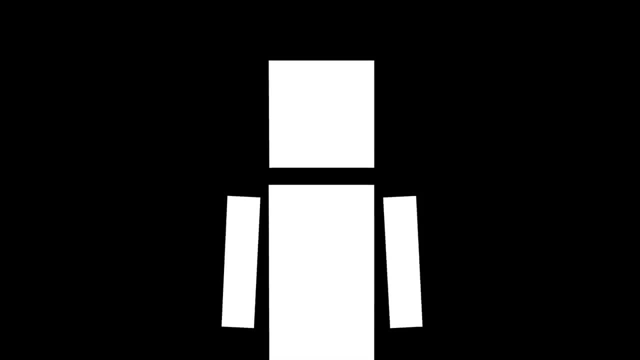 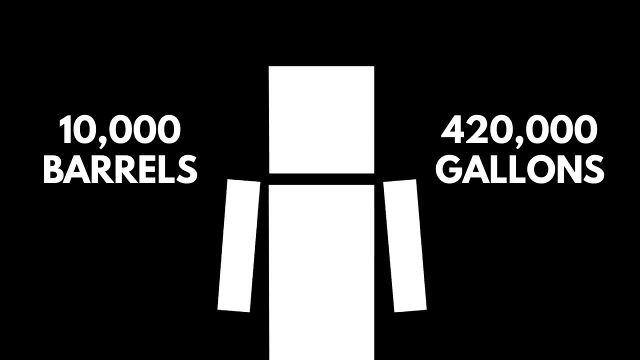 However, in the past 50 years or so, oil spills have been more common in the US than in the US than in the US, There has been over 44 oil spills, each over 10,000 barrels or 420,000 gallons of oil that have impacted US waters. These spills have 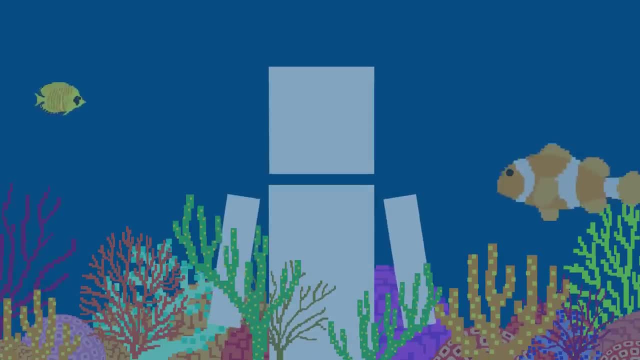 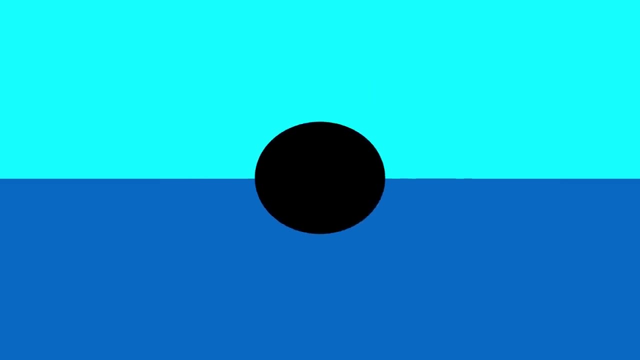 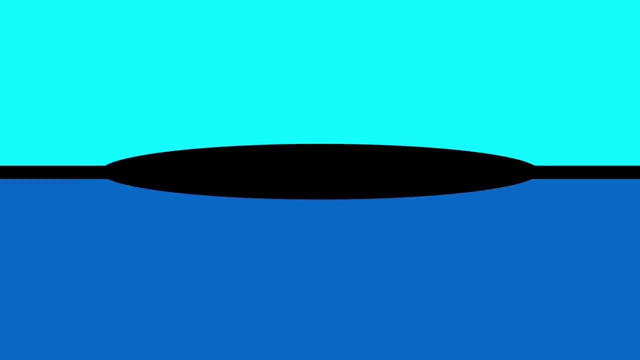 the potential to be very harmful to the environment, marine life and even humans. After a spill, since oil is less dense than water, it will typically float on the surface of the water. It doesn't just stay there in some big glob, though. What usually happens is that the oil will. 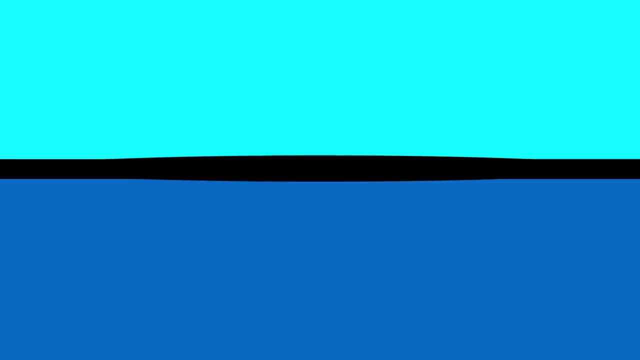 rapidly spread out over the surface of the water until it becomes a thin layer of oil known as an oil slick. Then it keeps spreading out until it forms a super thin layer called a sheen. But that thin layer of oil can be a big problem.